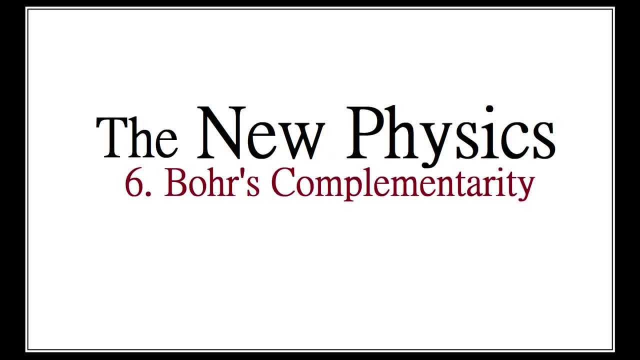 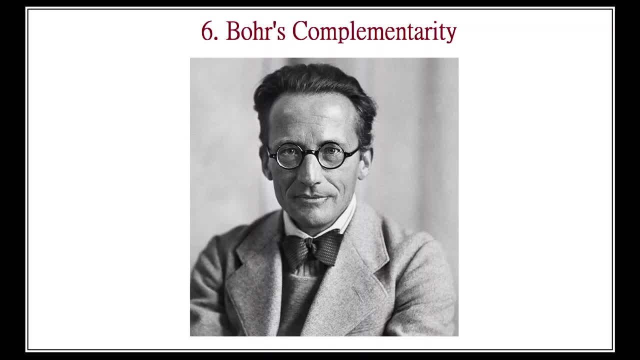 Needless to say, many physicists were not happy with this quantum predicament. Schrodinger, for instance, had assumed his equation was just a temporary fix, something to hold us over until we had figured out what is really going on down there. Most everyone assumed that there has to. 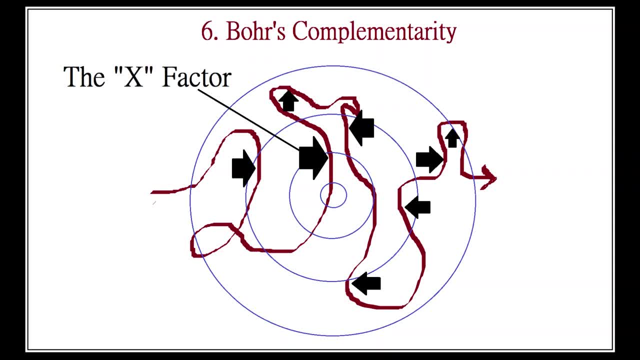 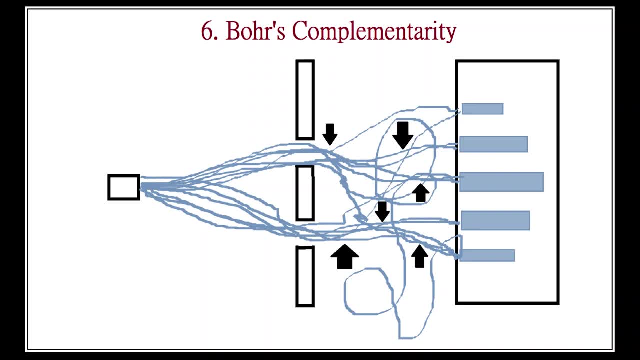 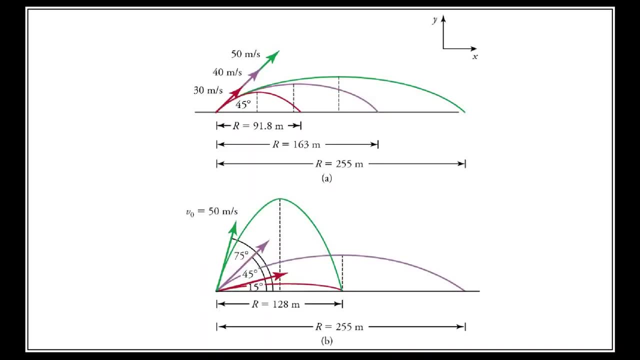 be some hidden variable influencing the motion of the photon. It can't literally be a wave while it's moving. It must just be moving in a way that appears either prescient or like it is covering all the possibilities. But once we discover some new force of nature or some new equation, we'll figure. 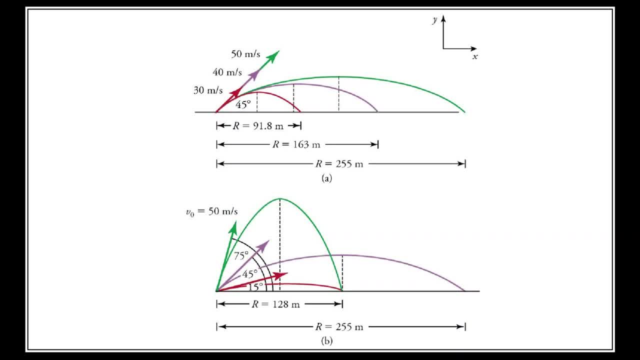 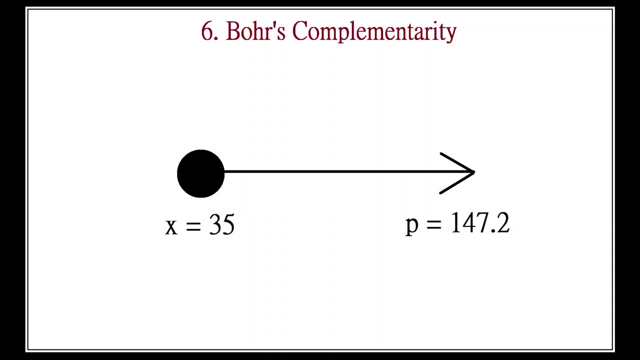 out how to track each photon individually and know why it landed precisely there and not there, just as we supposedly do with cannonballs and bullets on the macro level. In other words, we'll overcome Heisenberg's uncertainty principle and be able to calculate a photon's momentum and position simultaneously for any 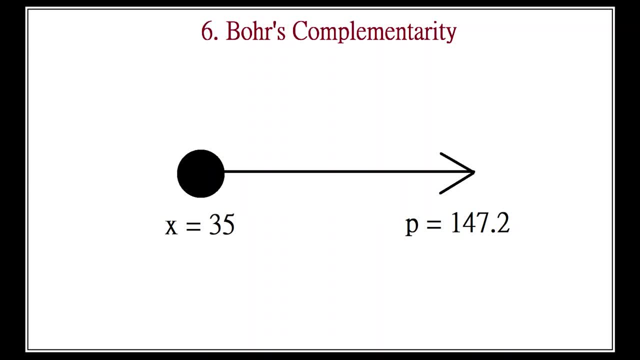 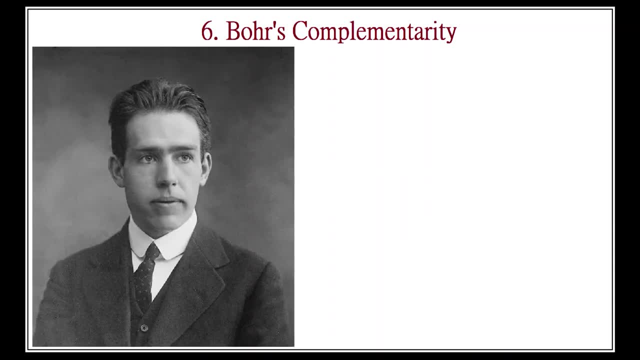 given point in time. There was one physicist, however, who did not believe this would work: Niels Bohr. He argued that there are no hidden variables. Quantum mechanics, as a mathematical description of the world is already complete. Probability and indeterminacy are sewn into the 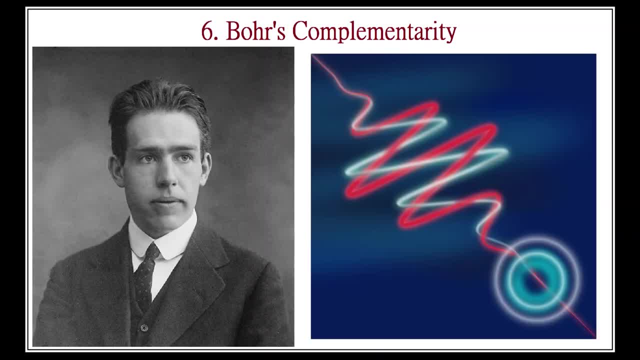 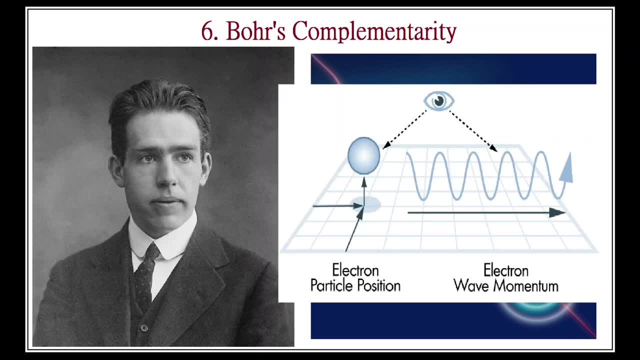 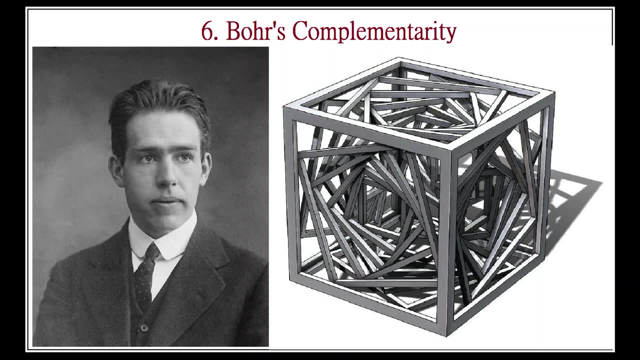 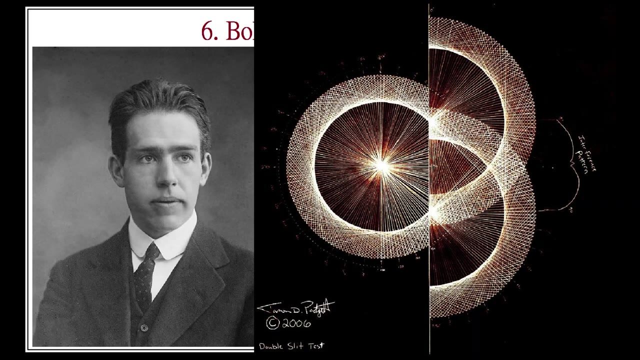 fabric of the universe, Because photons are both waves and particles. yet we, as observers can only see one of these states at a time. Reality is more complicated than any single model can account for or experimental apparatus can detect. Instead, we have to switch between two models to see the whole picture. 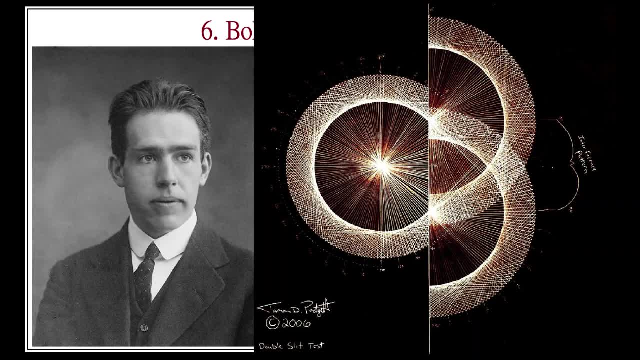 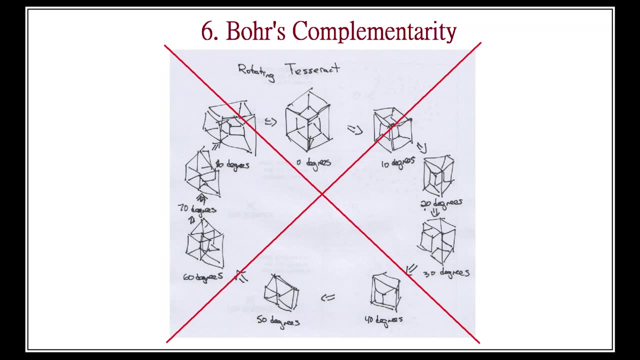 like using two synonyms to better describe the same object, or mixing two languages to better convey one's meaning. It is essential to understand that this is not because we haven't just invented an experiment or model that could capture the whole picture at once For Bohr. 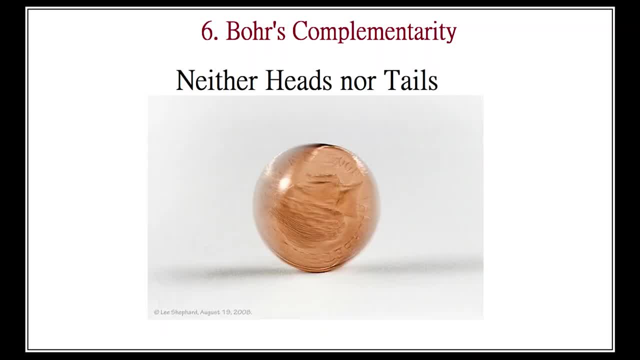 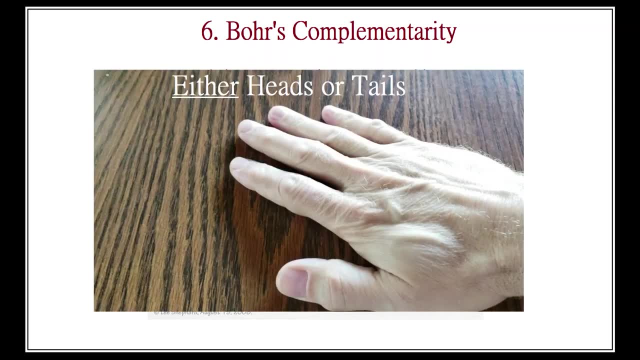 when we measure something, we are not discovering a reality that was there all along. Rather, our measurement actually determines a previously indeterminate reality. Measurement, in a sense, creates reality, Or rather causes reality to create itself in order for it to interact with the measuring. 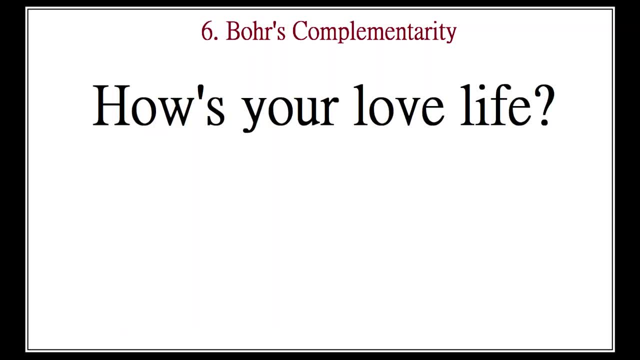 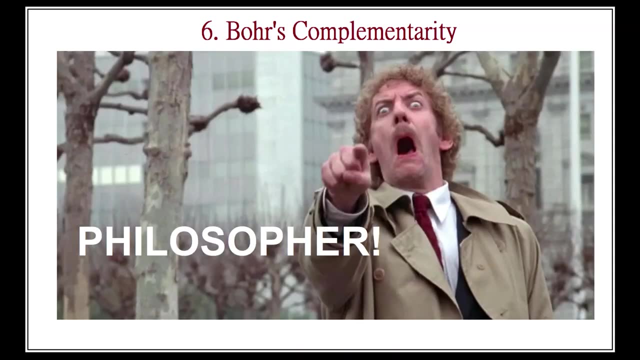 apparatus that we put in its way. We ask it a question, and the manner of the question that we ask forces it to respond to us in a particular way which reveals some things but shields other things from our view. Bohr's approach is often labeled idealist or even anti-realist. This is 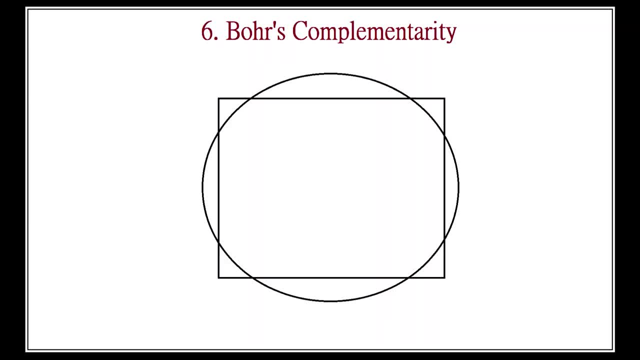 painfully ironic, because Bohr's approach is often labeled idealist or even anti-realist. Bohr's whole point is that reality cannot be perfectly contained within the human mind. For Bohr, reality is independent of our minds in a far more radical way than most physicists. 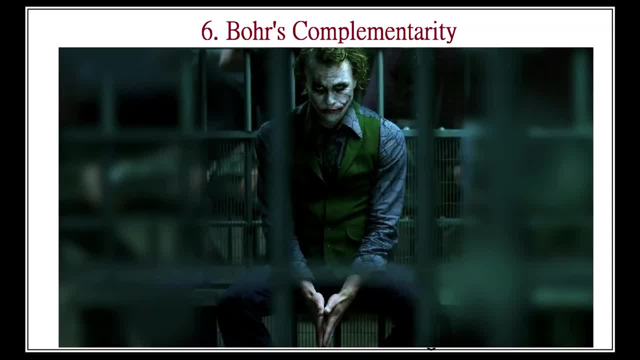 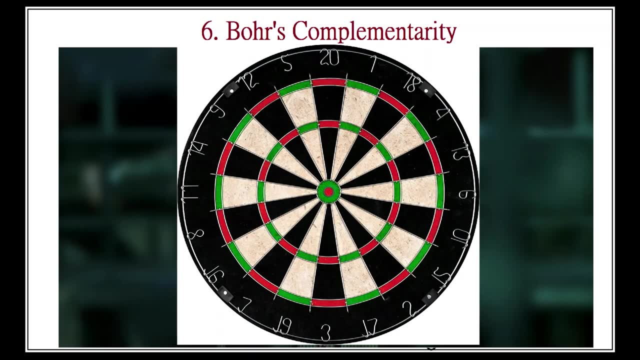 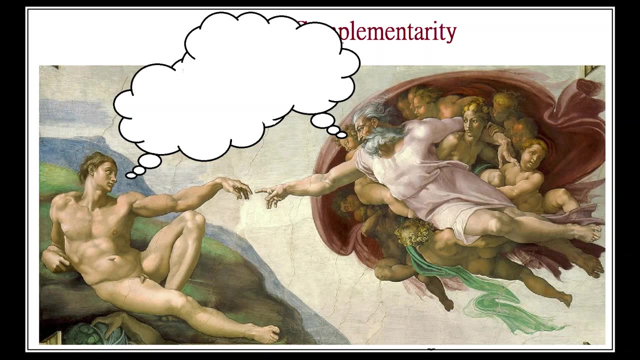 are actually comfortable with. It is so independent that we cannot predict what exactly it will do, But with the use of complementary models we can approximate what it will do in different situations. Bohr described Einstein's ambition to quote know the mind of God with his famous retort: 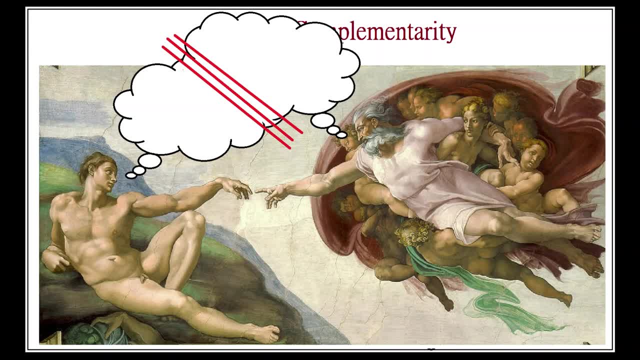 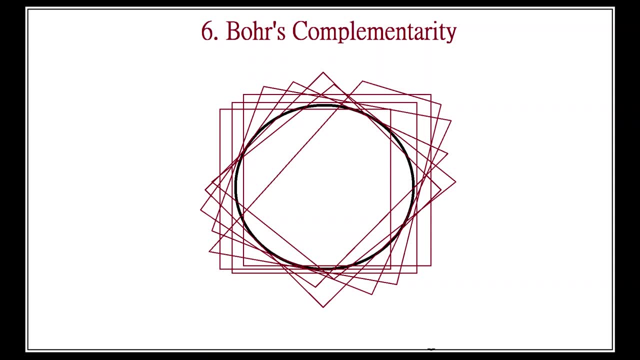 don't tell God what to do. God's thoughts are not our thoughts. Our words, models, mathematics and even our actual experiments cannot pigeonhole reality, which transcends the dualities through which we are ordained to comprehend it. Bohr referred to this idea that mutually exclusive. 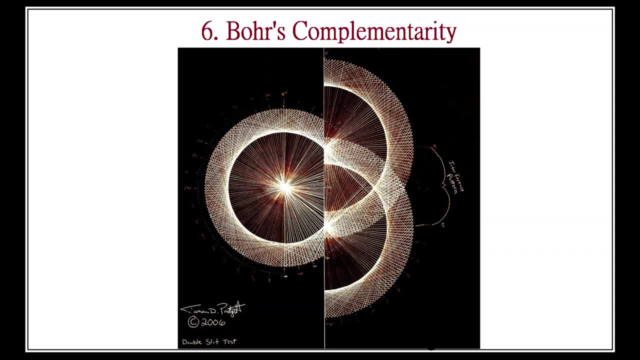 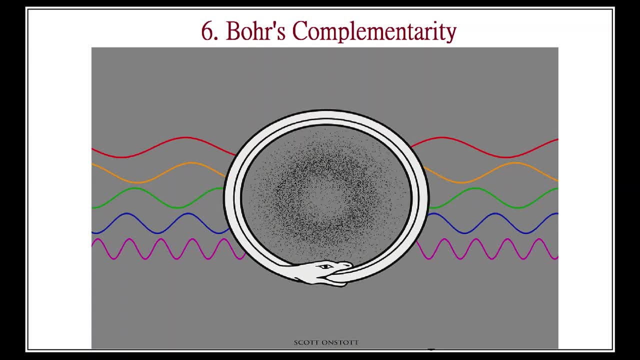 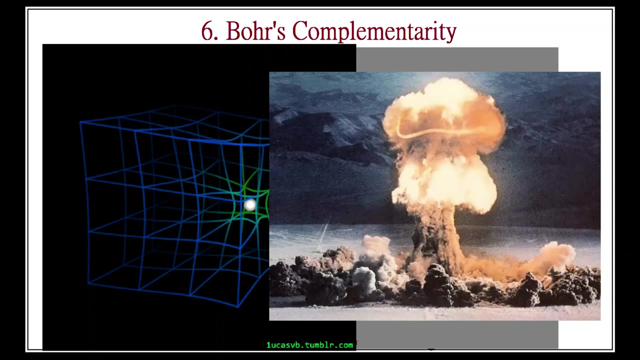 models are necessary to quote, fully describe the same thing as complementarity. The wave model and the particle model complement each other in describing a living reality which transcends them both. Bohr argued that we do the same thing with many other concepts- space, time and mass energy, for example- And he suggested on 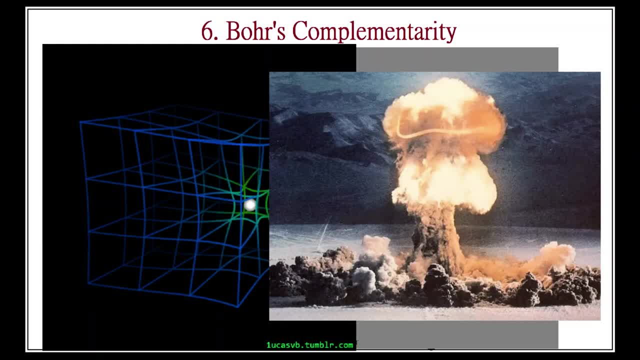 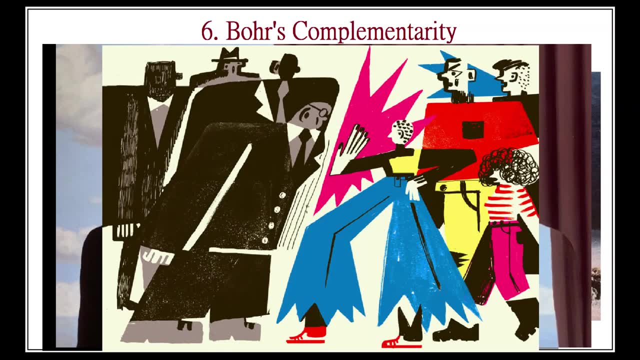 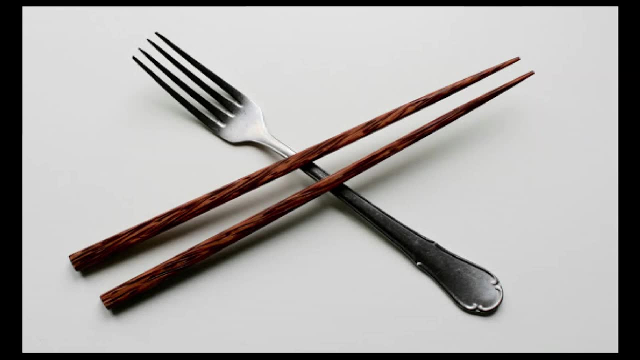 many occasions that this idea of complementarity could just as well be applied to science versus religion, body versus mind and even culture versus culture, in the sense that different cultures could be treated as complementary approaches or solutions to the problems of human life. In this sense, Bohr was a. 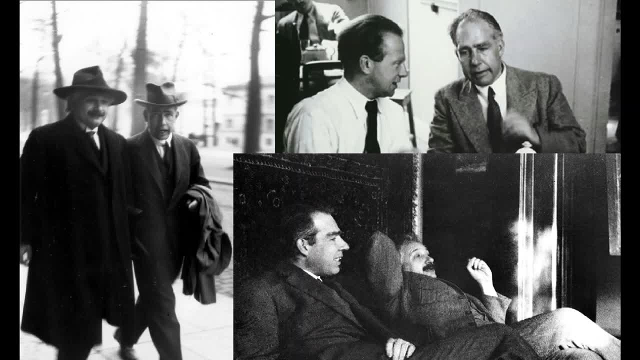 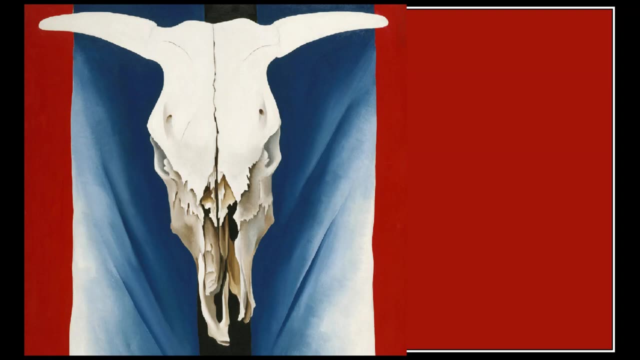 reconciler, who wanted to find the value inherent in all things and was not interested in setting worldviews against each other in a tournament of dominance. So much for Bohr's theory of the universe. 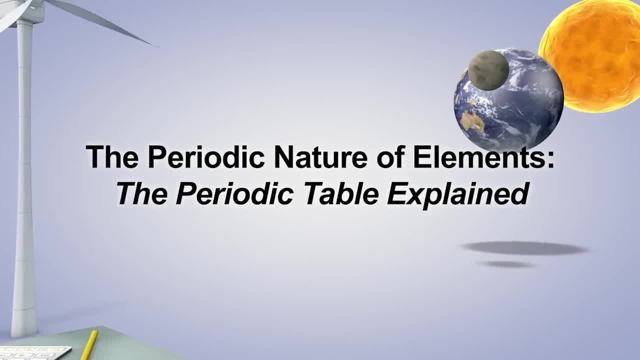 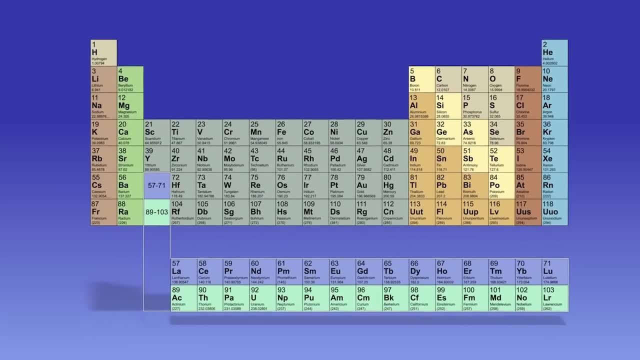 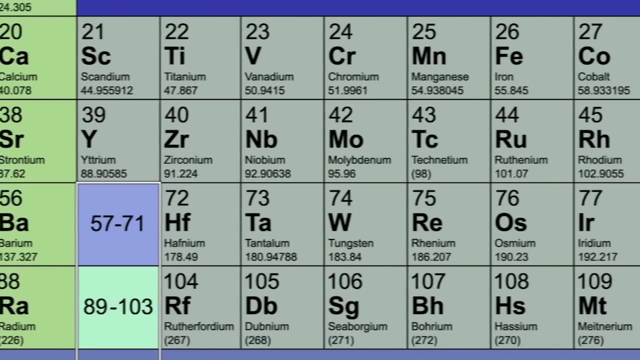 The Periodic Nature of Elements. The Periodic Table Explained. Although the Periodic Table of Elements looks complex, it is easier to follow once you learn how to use it. First, the letters are symbols. Each box represents an element. Each element is made up of the same kind of atom with a specific number of protons in its nucleus. 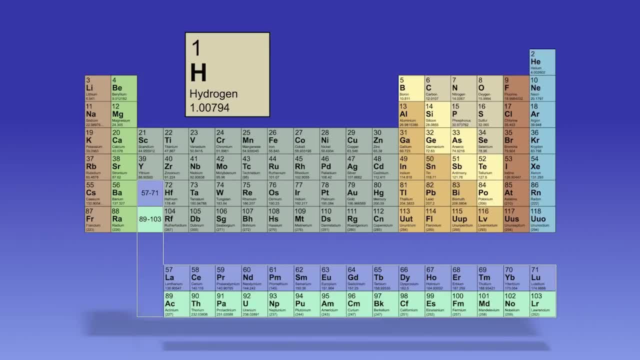 the atomic number. For example, H represents hydrogen. All hydrogen atoms have one proton. The symbol HE represents helium. All helium atoms have two protons. The elements are arranged by increasing atomic number. The atomic number displays how many protons are present in the 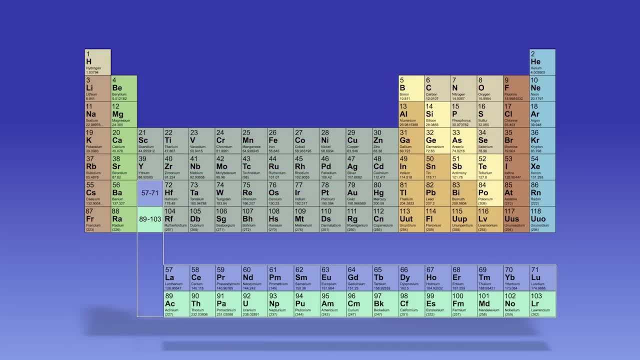 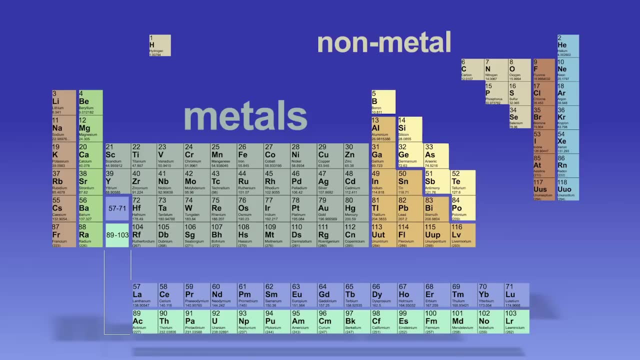 nucleus of the atom. The table is also very colorful. Each box is color-coded to show whether the element is a material or not, The number of protons in the nucleus of the metal or non-metal, indicating the specific type. If you take a closer look at one element in particular, 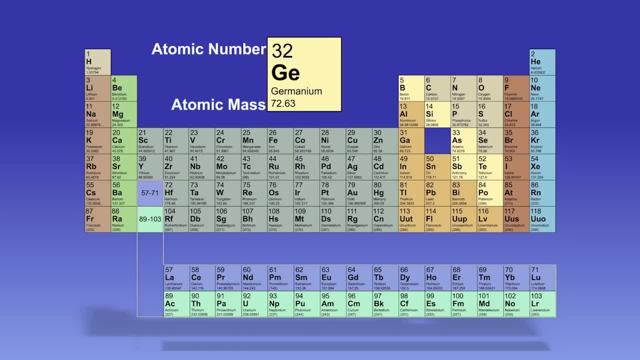 you will find its atomic number, atomic mass, element name and element symbol. Looking at the overall table again, you will notice that it is made up of columns and rows. The columns are known as groups and the rows are known as periods. 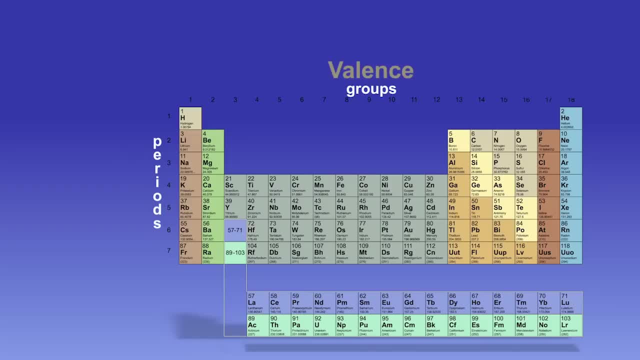 All elements in a group have similar characteristics. These characteristics will tell you how many valence electrons- the electrons in the outer shell of the atom- are present in that atom, giving you an idea about how they bond. Here are the element groups and the number.